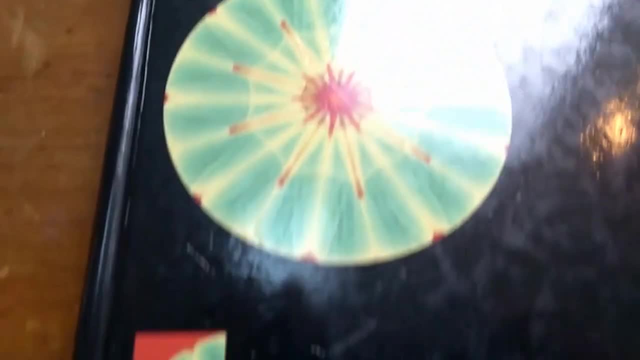 It's called Contemporary Abstract Algebra, and the author is the famous Joseph A. Galleon. So this is a fantastic book, and let's talk a little bit about it. 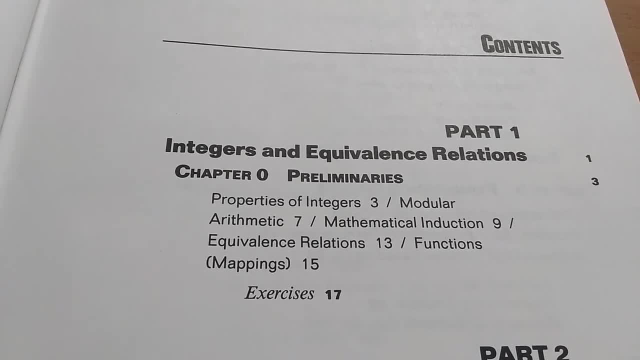 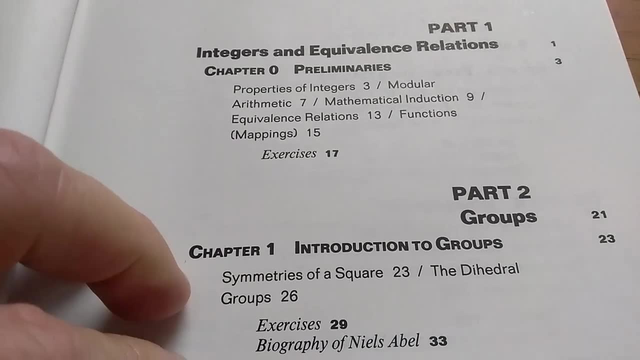 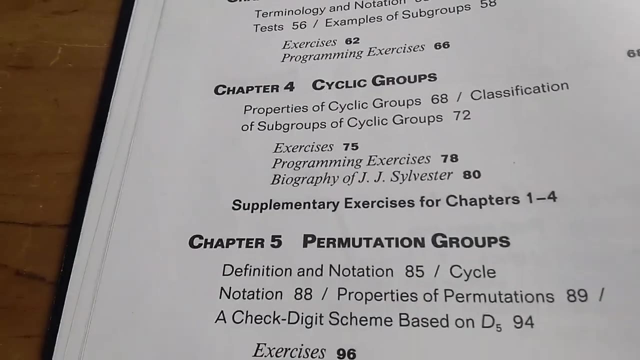 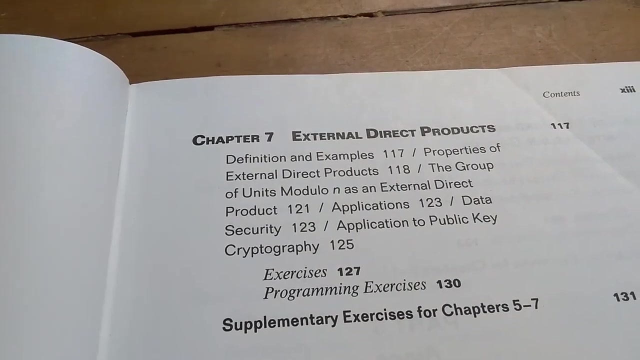 So first, let's briefly go through the table of contents. So it starts off with integers and equivalence relations. Then it goes on to groups. Let's see what's on the next page. More on groups, finite groups and subgroups, cyclic groups, permutation groups, isomorphisms, so pretty standard. Direct products, he specifically calls them external direct products. Cosets and Lagrange's theorem. Normal subgroups and factor groups. 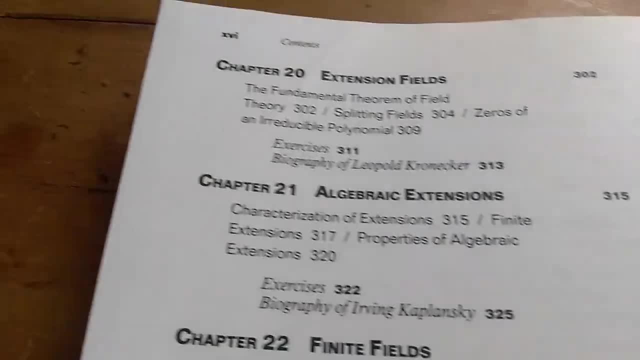 Group homomorphisms, and let's see if there's more. Let's see. I skipped some stuff. 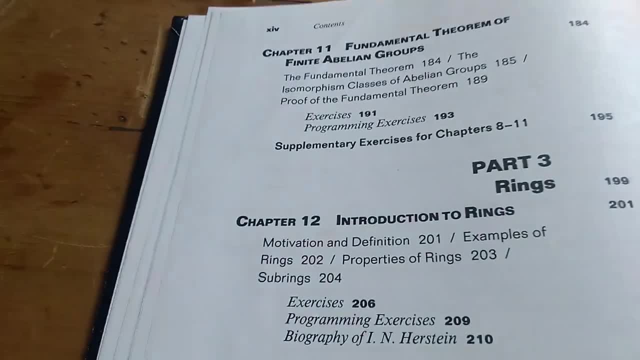 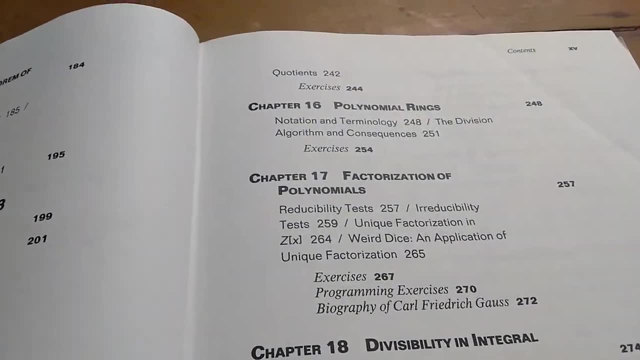 There's more stuff here. Fundamental theorem of abelian groups. Wow. Introduction to rings, integral domains, ideals and factor rings, ring homomorphisms, polynomial rings, factorization of polynomials, divisibility and integral domains. 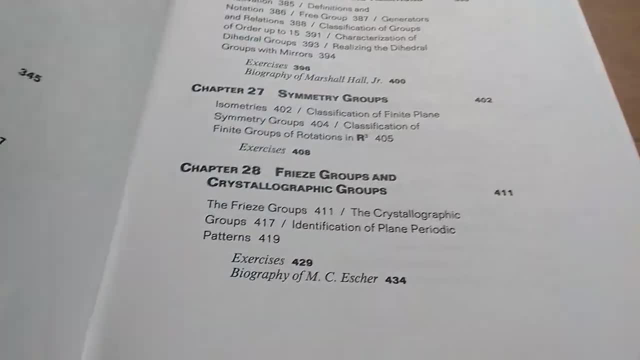 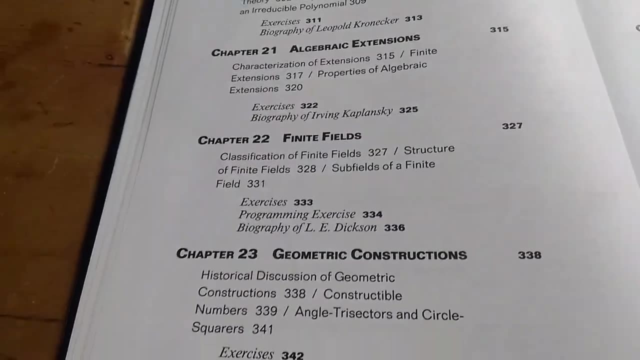 And then part four is on fields. Talks about vector spaces. Wow. A lot of information in this book. Extension fields, algebraic extensions, finite fields, some geometric constructions. Then in part five, he goes into the SELO theorems. And so like some more stuff. 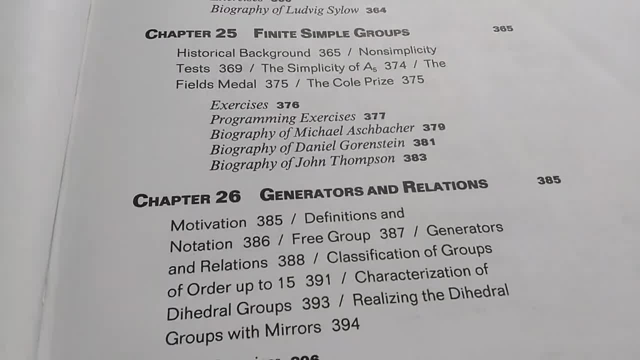 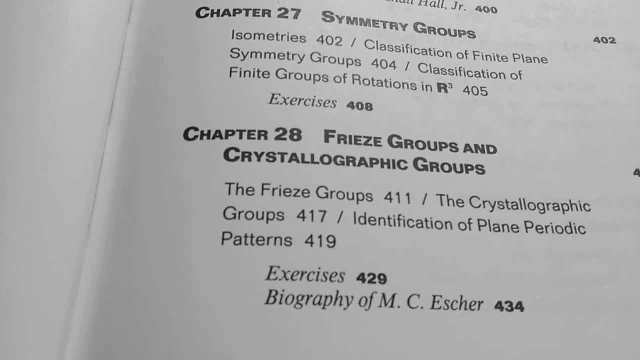 Specialized group theory, finite simple groups, generators and relations. And some stuff here on freeze groups and crystallographic groups. I don't know what those are. I've never looked into that stuff. 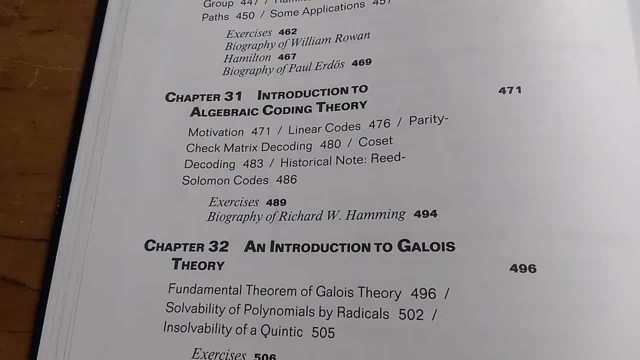 Goes into symmetry and counting, some Cayley digraphs and some coding theory. And at the very end, talks about Galois theory. So tons of information in this book. So I have personally found this book useful. 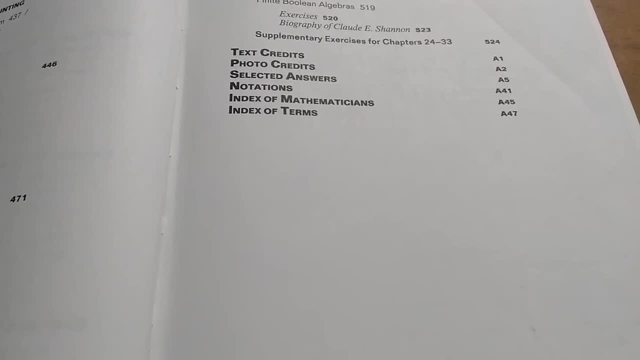 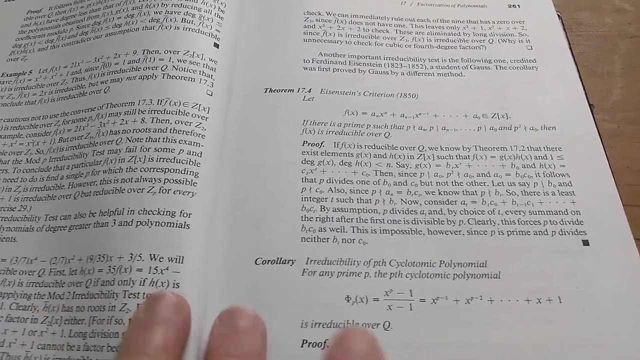 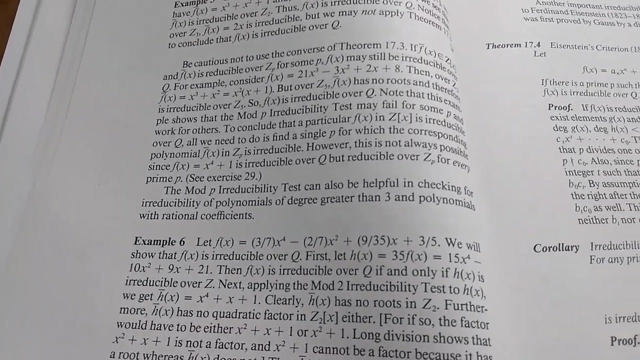 For some specific things and let me show you what those are. So I think the most useful thing I have found in this book and the thing that sticks out about this book the most are the examples. This book has a lot of examples that other books do not have. So whenever I think of Galleon's book, I think of it as a book that has a lot of examples of things that you cannot find in other books. 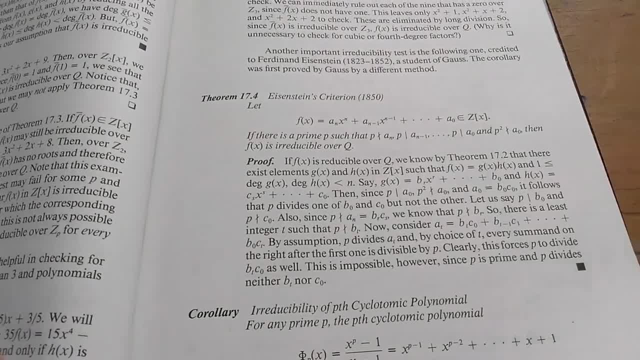 So I think this is a good book. I think it serves as a good supplement to other books. 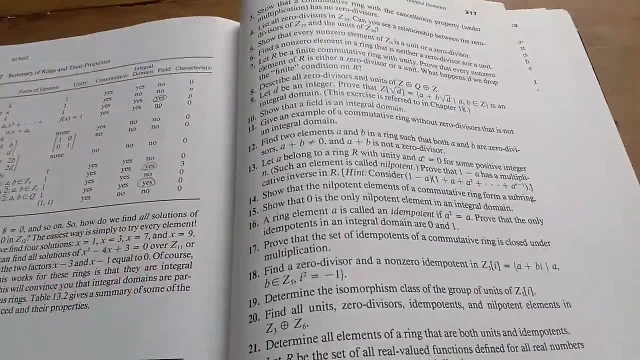 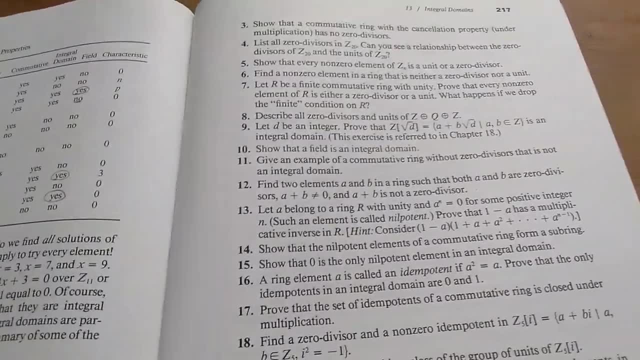 You could probably teach yourself abstract algebra with this book together with some help from the internet and other books. The problems in this book are pretty good. I think there are solutions to the problems. Yeah. 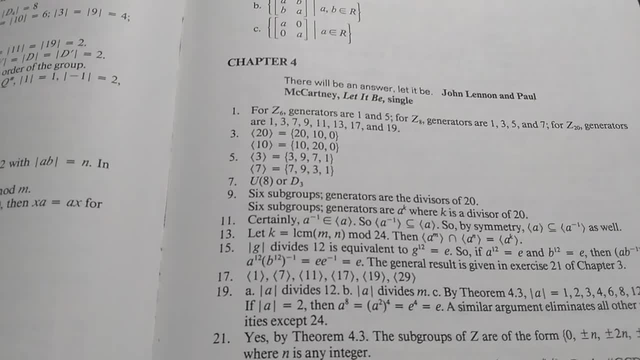 So a lot of the problems have partial solutions or solutions which is beneficial. 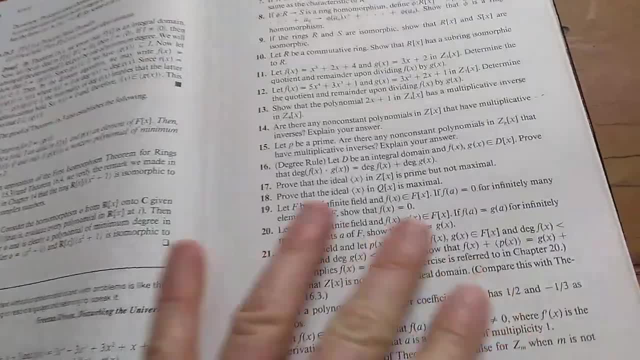 But again, for me personally, I have mainly used this book as an additional source of knowledge. And specifically, I have found it useful. 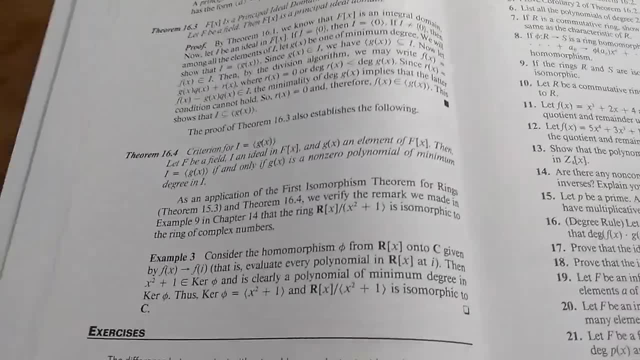 I have found the examples in this book to be really helpful. So it's a good book.